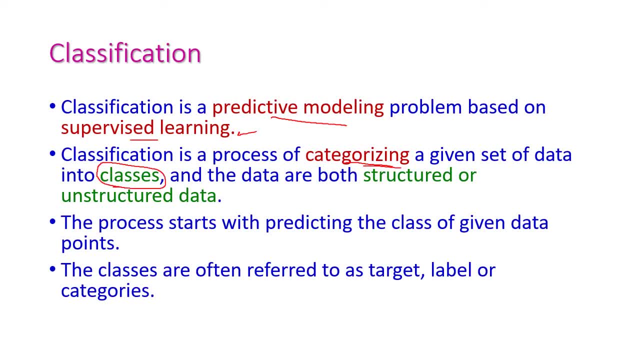 and the data are both structured and unstructured data. Okay, we know what is structured data and what is unstructured data, So the given data will be categorized into number of classes and the process starts with predicting the classes of given data points and the classes. 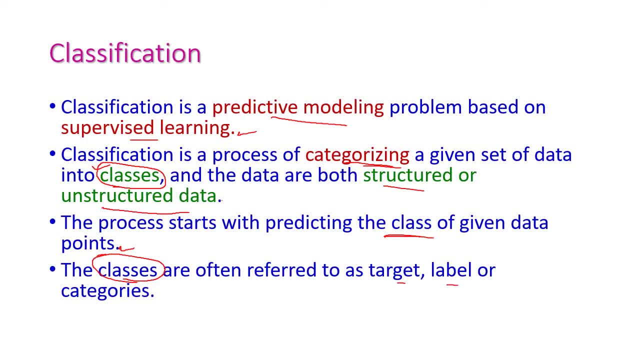 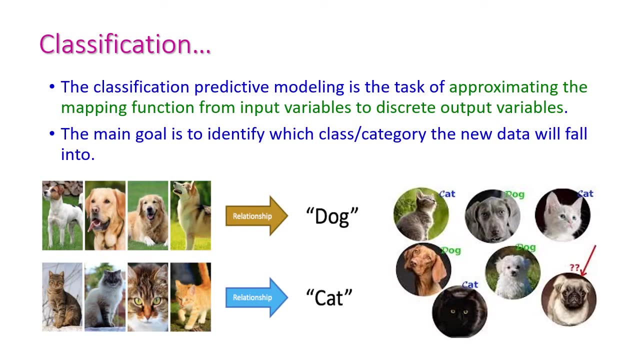 are referred as the target label or categories, So this is called as classification. What is classification? Classification is going to classify the given set of data into different, different classes. Classification is a task of approximating the mapping function from input variables to 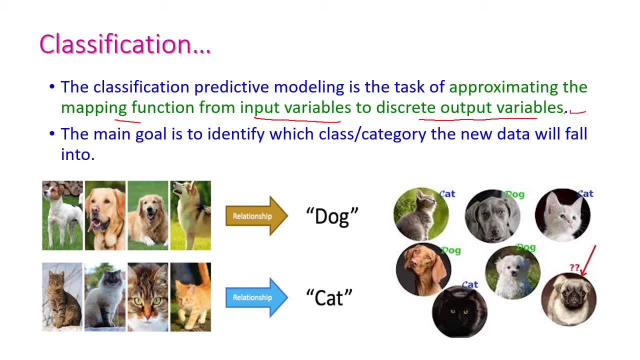 discrete output variable, and the main goal of this classification is to identify which class or category the new data will fall into. Okay, here, in this example, we are having a set of data that belongs to the class dog and another set of data that belongs to the class cat. 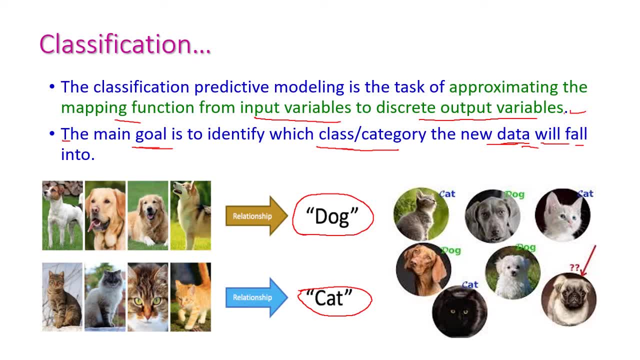 Okay, and now? what is our goal? We need to identify which class or category the new data will fall into. Okay, so here these are the data that will come to our classification problem, and all the data are having its own label. Okay, so the first one is cat. that will belongs to this class. cat, Okay. dog, dog will belongs to this dog class. 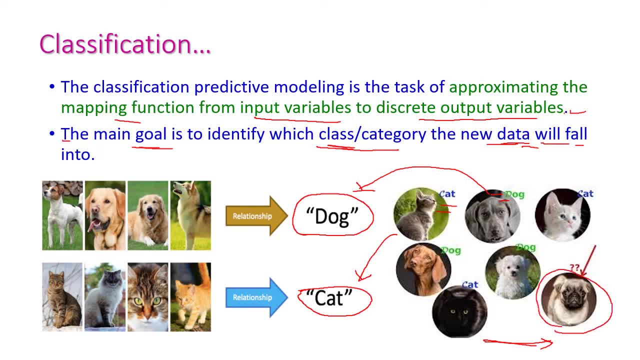 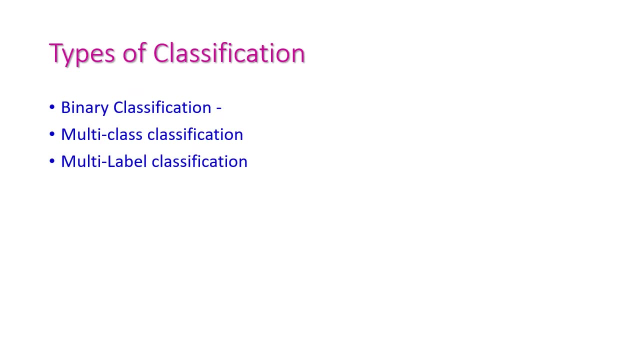 Okay, likewise, and now we need to predict what is this? This is a dog and this will come under the class dog. Okay, dog class. This is called as classification, and we are having three different types of classification. First one is binary classification. 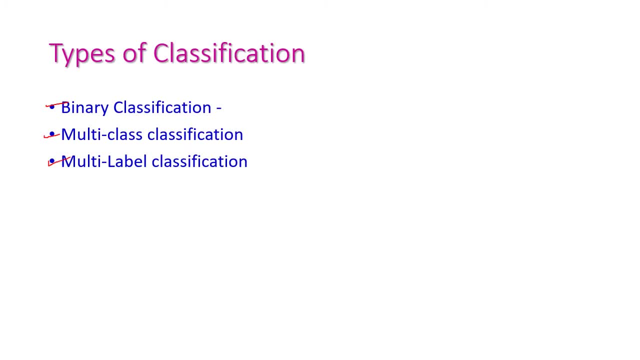 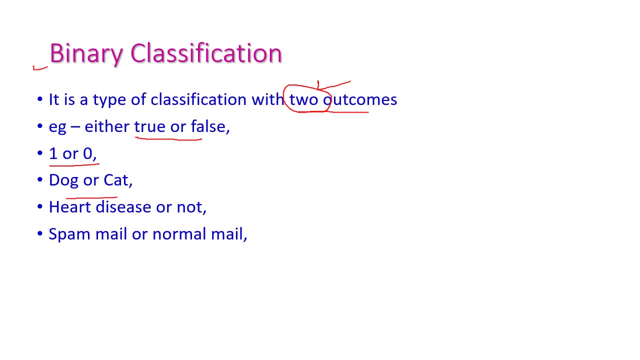 Second one is multi class classification. multi class classification and multi label classification. Let us see all these things one by one. The first one is binary classification. So in the binary classification the output or the outcomes will be only two, Only two. It may be either true or false, Zero or one, Dog or cat, Heart disease or not, Spam mail or normal mail. 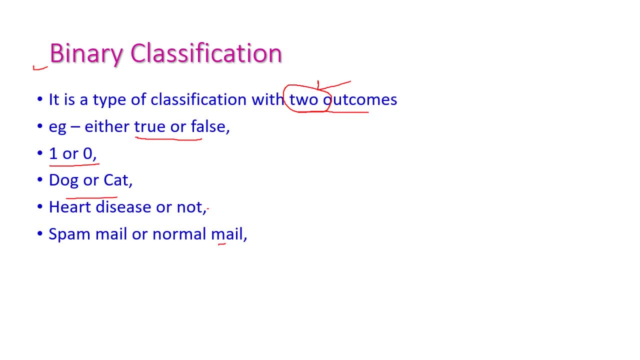 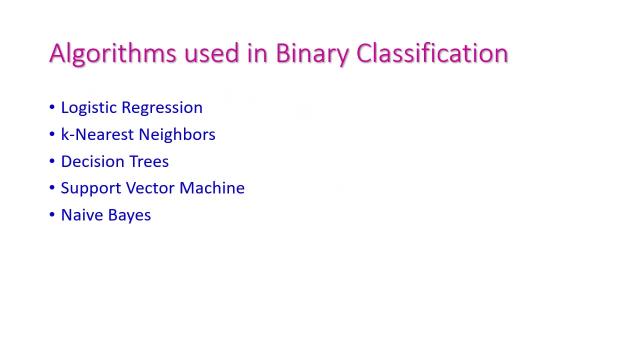 That means it will predict, predict only any of these two classes. the classes, output classes, will be only two. okay, this is the first class and this is the second class. all the given input item will belongs to any one of this particular two classes. so this is called as binary classification right and the algorithms used in 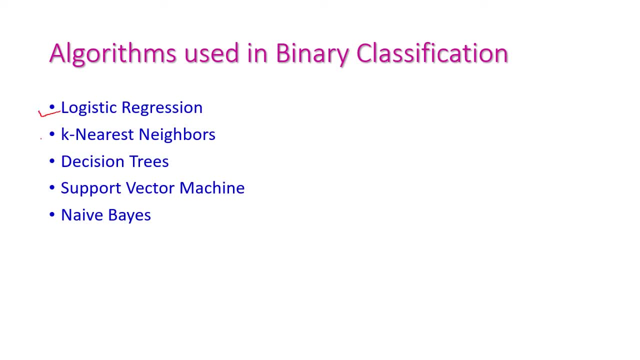 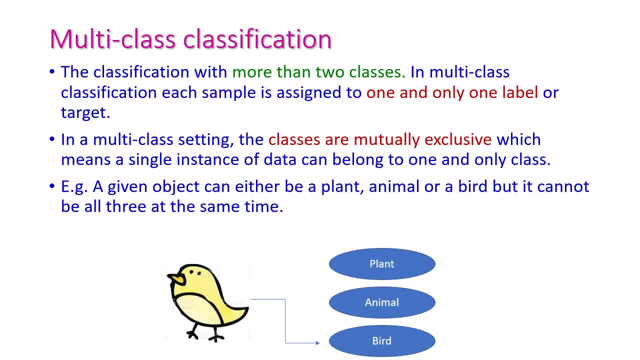 binary classification are logistic regression, k, nearest neighbors, decision trees, support vector machine- that is, svm- and naive base. so these are the popular algorithms that will come under binary classification. the next one is multi-class classification. in this multi-class classification we are having more than two classes, more than two classes, and here each sample is: 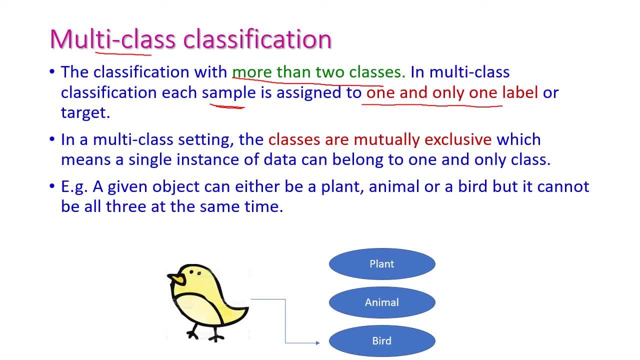 assigned to exactly only one label or only one target, so this is called as multi-class classification. more than two classes are there. more than two classes are there, but the incoming incoming sample will be assigned to any one of the class, not both. the classes are all the classes at. 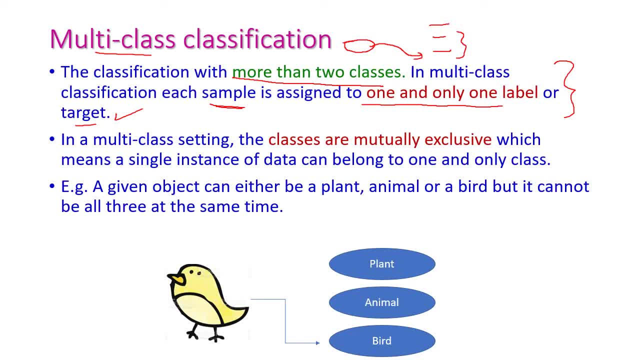 a time. okay, so this is called as multi-class classification. here all the classes are mutually exclusive. the classes are mutually exclusive. that means a single instance of data can belongs to only one class at a time. okay, let us see one example for this. so given an object is either plant, animal or 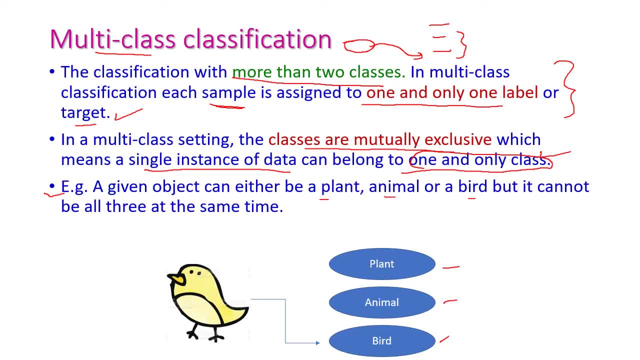 bird. this is our problem here. we are having three different classes: plant class, animal class and bird. now we are having an input data. this is our input data. which belongs to which class? the bird class? isn't it this particular bird that should be assigned to bird class? but this should not be. 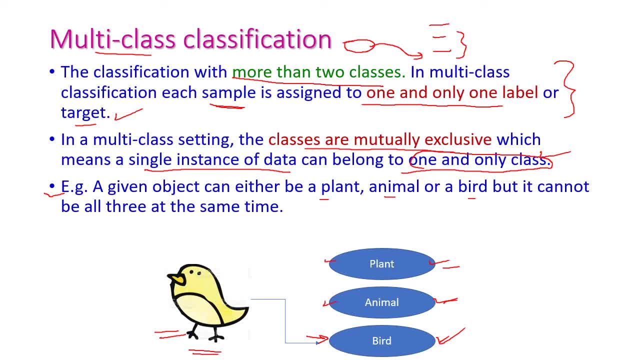 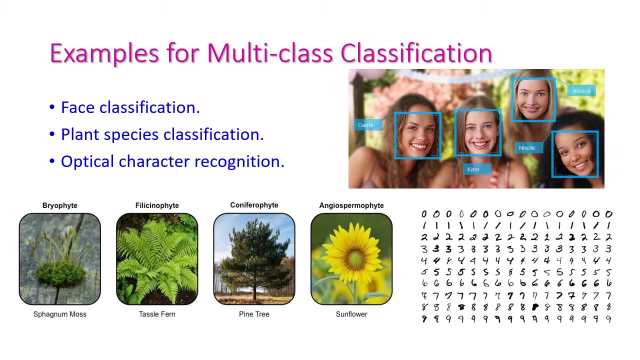 assigned to any of this animal class or plant class. okay, so the input should be assigned only one class at a time is called as multi-class classification. and let us see some examples for multi-class classification. first one is face classification. so this is the very famous example which is taken from facebook. okay, so four different peoples are there wherever we upload this particular image, and this name should be the same. okay, so this particular data will be assigned to only this class. and let us see some examples for multi-class classification. first one is face classification. so this is the very famous example which is taken from facebook. okay, so four different peoples are there wherever we upload this particular image, and this name should be the same. okay, so this particular data will be assigned to only this class. and let us see some examples for multi-class classification. first one is face classification. so this is the very famous example which is taken from facebook. okay, so four different peoples are there wherever we upload this particular image, and this name should be the same. okay, so this particular data will be assigned to only this class. and let us see some examples for multi-class classification. first one is face classification. so this is the very famous example which is taken from facebook. okay, so four different peoples are there wherever we upload this particular image. 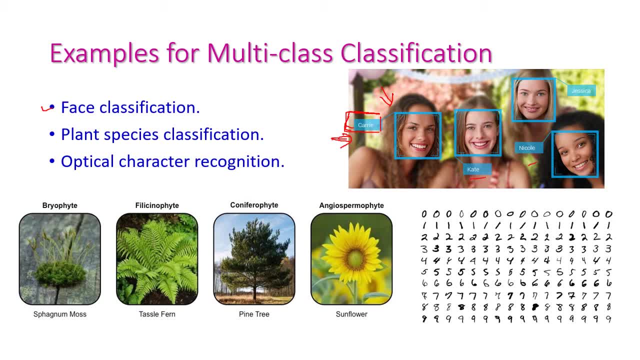 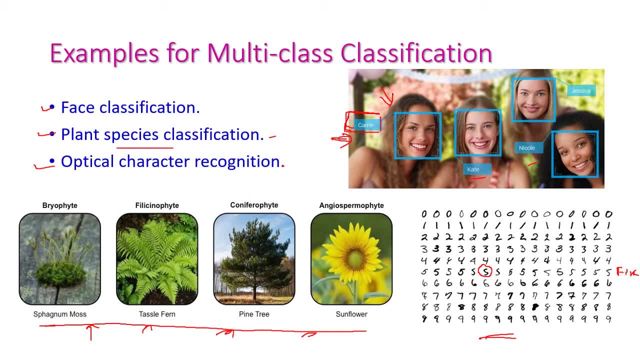 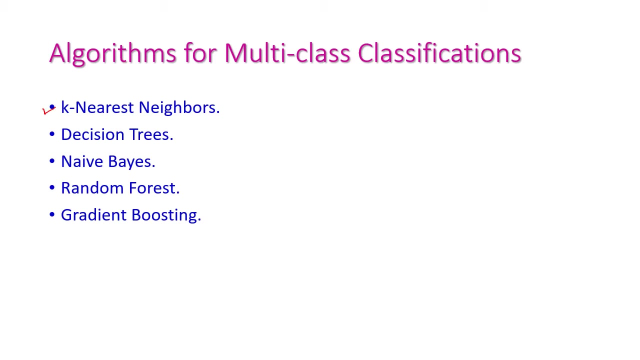 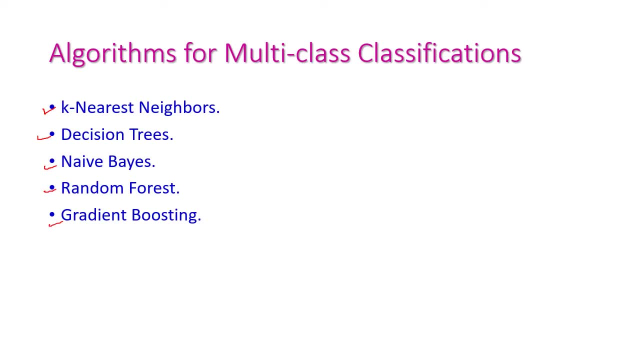 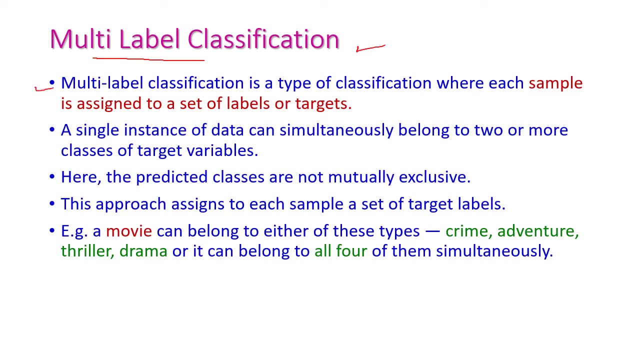 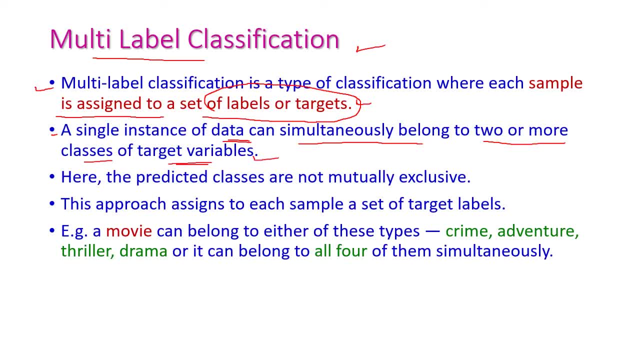 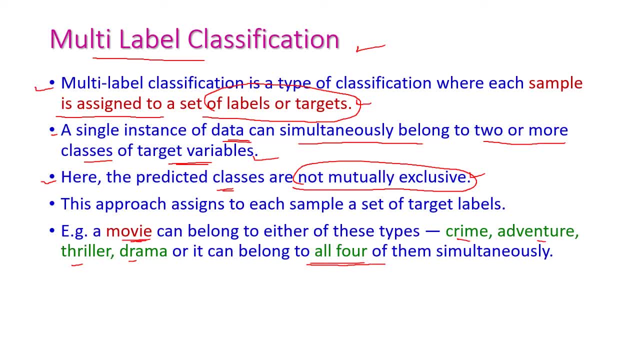 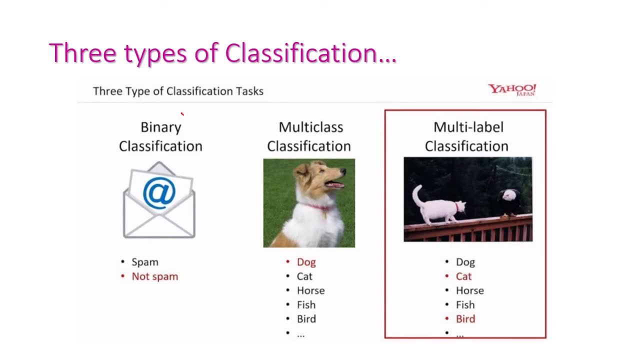 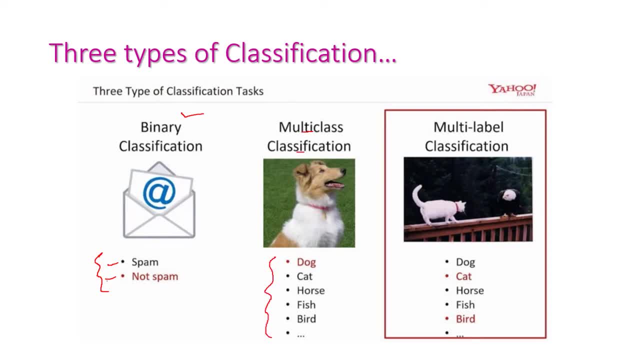 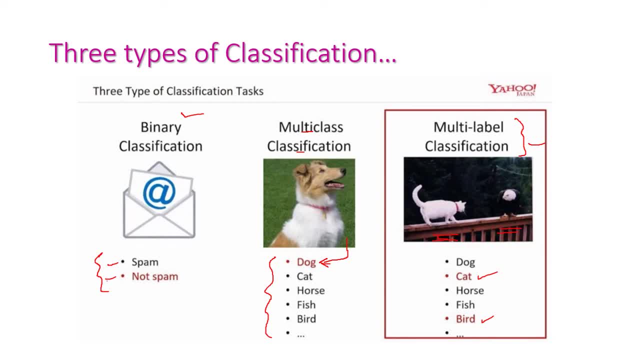 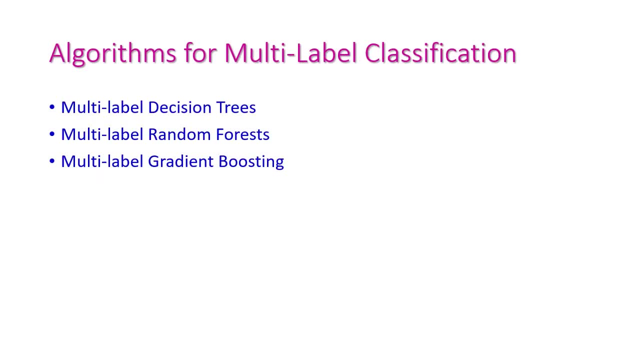 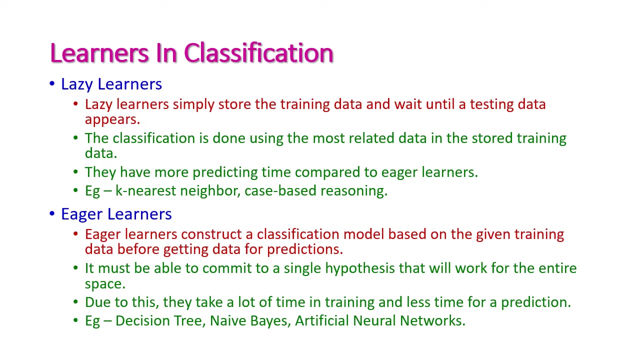 classes cat and bird. okay, so this is multi-label classification, and the popular algorithms for multi-label classification are multi-label decentry, multi-label random forest and multi-label gradient boosting. and there are two other categories of classification: first one is lazy learner and second one is eager learner. okay, that is learners in classification. 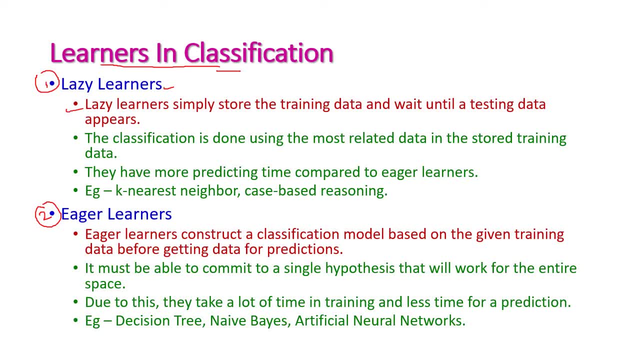 what is lazy learners? lazy learners are simply store the training data and wait until the testing data appears. it will accept the training data and it will wait until the testing data will come. okay, the classification is done using the most related data in the stored training data and they have more predicting time. they 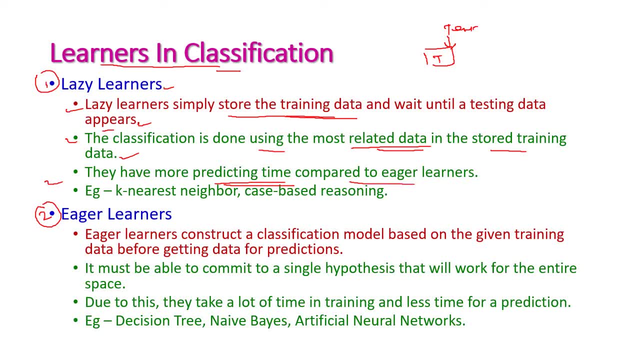 have more predicting time when compared to eager learning, that is, it will take more time for train itself. for example, k: nearest neighbor and case based reasoning are the popular algorithms for lazy learners, and next one is the eager learner. okay, so eager learner is the classification model based on the given training data before getting the data for prediction. 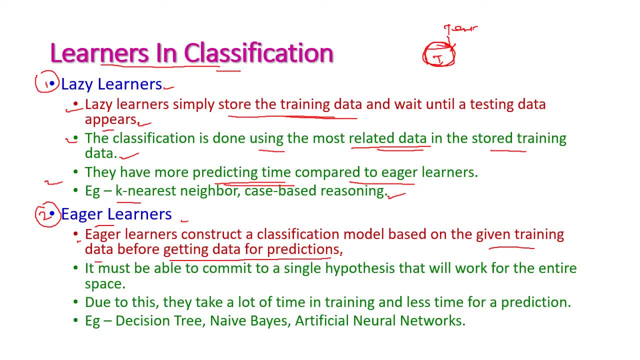 itself. so once it gets the training data, the learn the algorithm will start learn by itself. right, and it must be able to commit to single hypothesis that will work for entire space and due to this, they take lot of time in training. lot of time in training and less time for prediction. 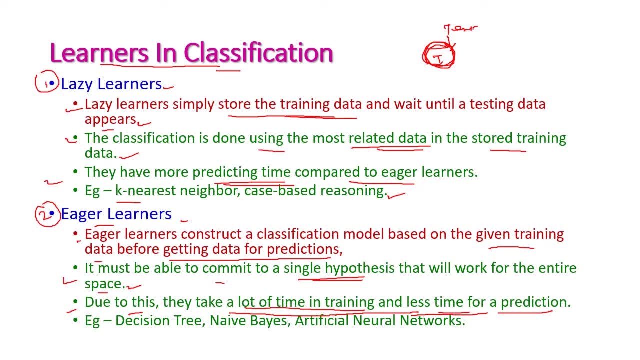 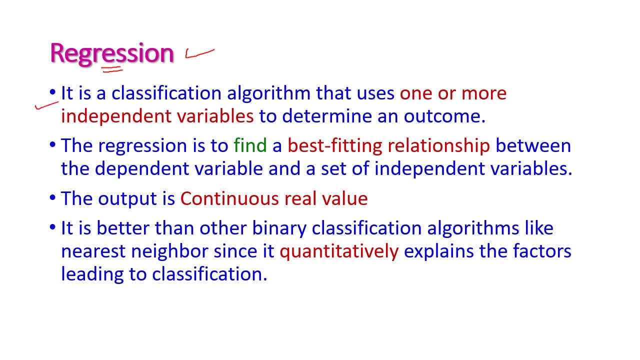 okay, and the popular examples for eager learners are decision tree knife base algorithm and artificial neural network. next we will move to regression. so it is also a classification algorithm that uses one or more independent variables to determine an outcome is called as regression. okay, regression is to find a best fitting relationship between the dependent variable and a set of. 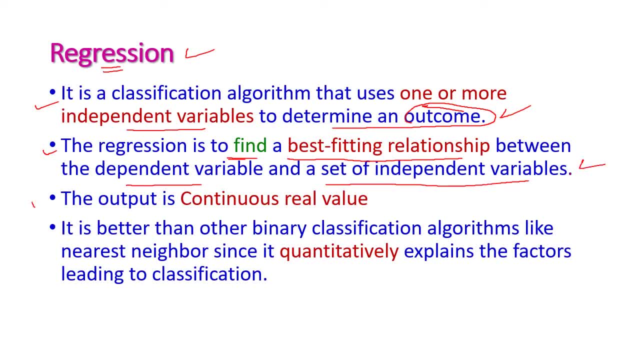 independent variables. the output is continuous real value. this is very important for regression. the regression output should be a continuous real value. so it is better than other binary classification algorithms like nearest neighbor, since it quantitatively explains the factor leading to the classification right. so in the classification the 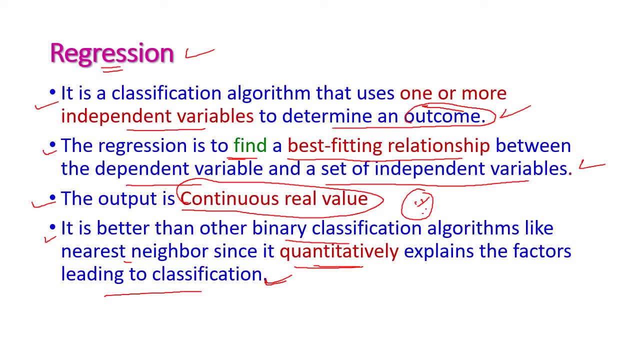 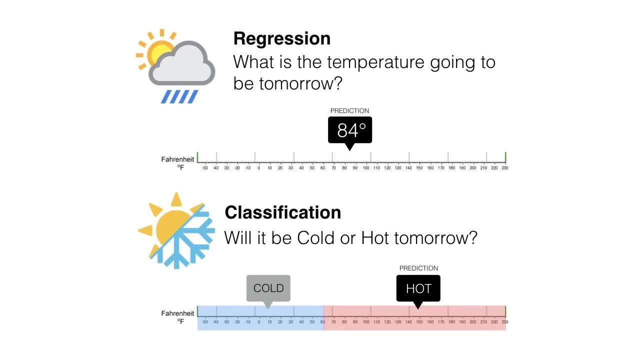 output will be any one of the classes, but when come to regression the output will be continuous real value. okay, so to predict the temperature for tomorrow. when come to classification, it will give either cold or hot it will give. the prediction will be either the climate is cold or the climate will be hot. so this is called as classification. but 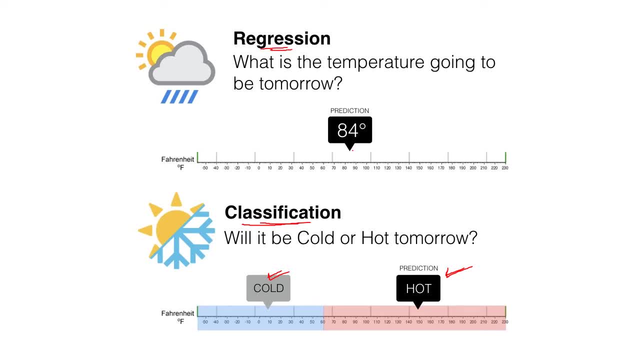 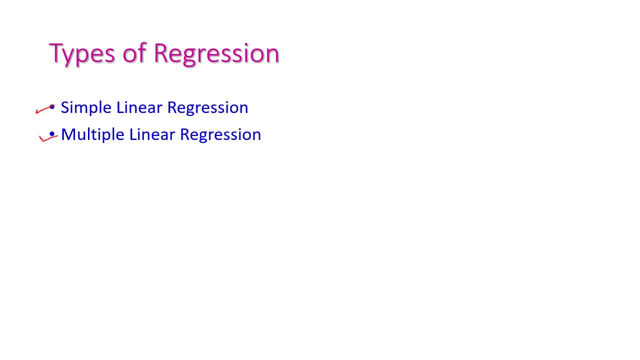 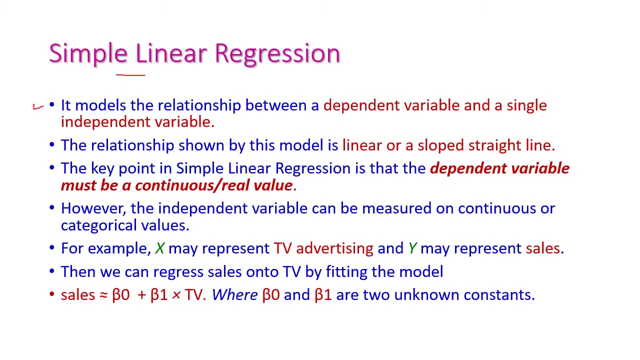 when come to regression, it tries to predict the exact temperature for tomorrow. so this is the difference between two tipo of authoritarian model, which isnik know the Choi, and some such classification and regressor. The type of regressor: The first one is simple linear regressor and multiple linear regressor. The first one is simple linear regressor. It models. 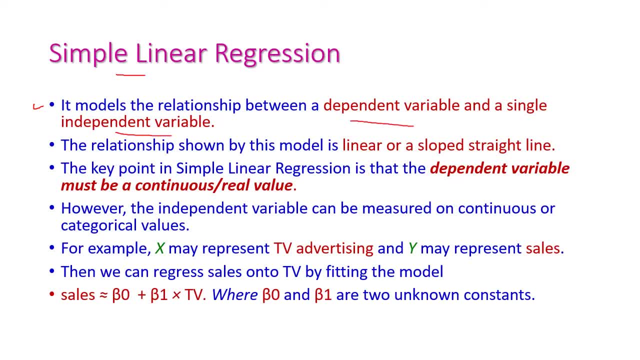 the relationship between dependent variable and a single independent variable. Right, So the relationship shown may be a straight line or a sloped straight line. Okay, The key point in simple linear regression is dependent variable. that must be a continuous or real value, The dependent variable. So this is the dependent variable That should be a continuous. 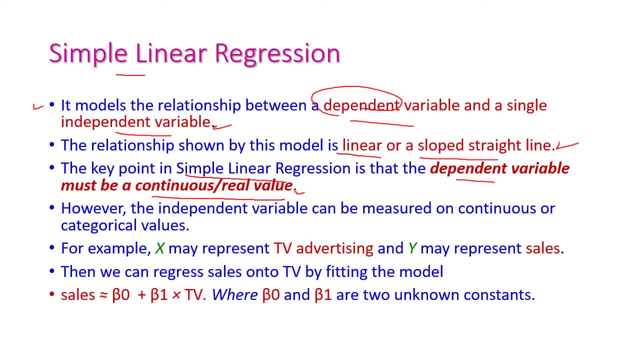 value or a real value, And the independent variable can be measured On continuous or categorical values. Right, For example, we can take X that represent TV advertising and Y represent sales. X is TV advertising and Y is sales. Then we can: 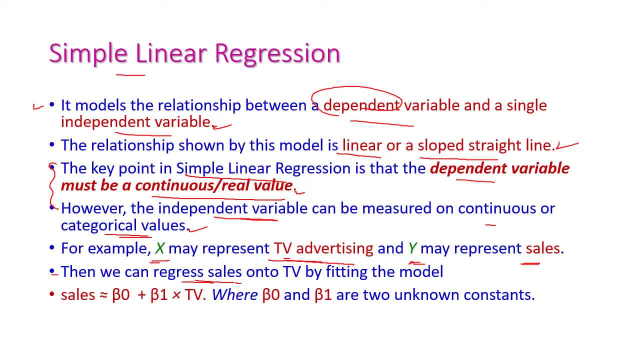 regress the sales onto TV by fitting the model Sales which is equal to. that is approximately equal to B Beta 0 plus beta 1 into TV, Beta 0 plus beta 1 into TV, Where beta 0 and beta 1 are two. 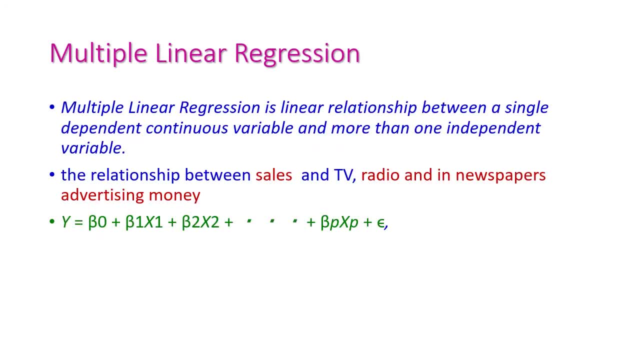 unknown constants. And the second one is multiple linear regression. Multiple linear regression means a relationship between a single dependent continuous variable and more than one independent variables. The dependent variable is only one and the independent variables are more than one. Okay, Now the relationship between sales and TV, radio and newspaper advertisement, Then Y. 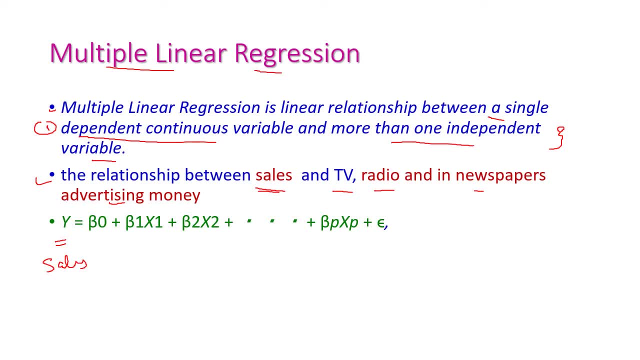 is equal to Y means sales. Sales, which is equal to beta 0 plus beta 1, X1 plus beta 2, X2, etc. plus beta P, XB plus E. This E means epsilon or error. Okay, So this is multiple. 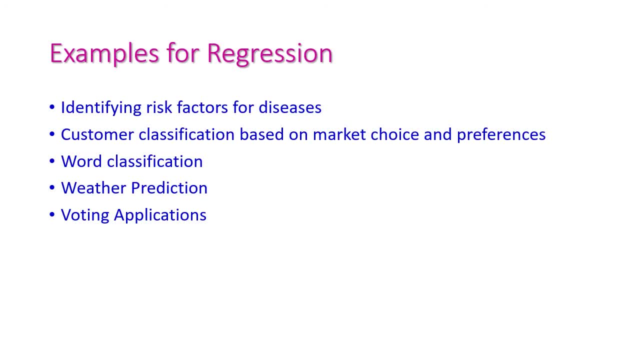 linear regression. Examples for regression Identifying risk factor for a disease. So in the classification that will give either we are having a disease or not, But in regression we are having a disease, But in regression that will give the risk factor of disease, How much disease? 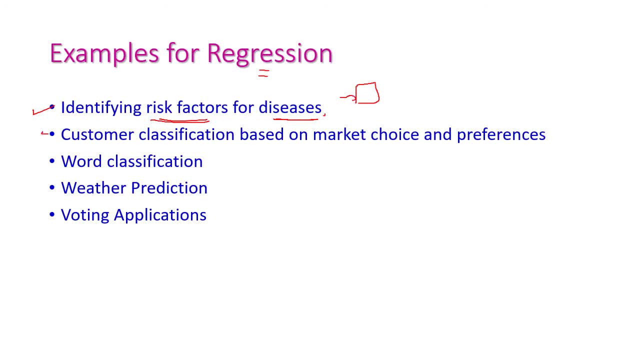 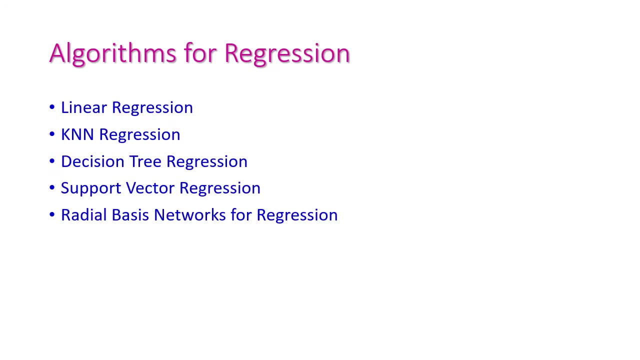 is there in your body Right. And next one: customer classification based on market choice and preferences, World classification, weather prediction, voting applications are some other examples for regression, And the popular algorithms for regression are linear regression, KNN regression, decision-making regression and linear regression. Okay, So these are the 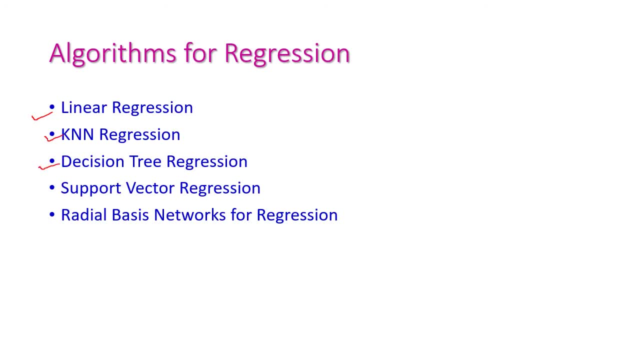 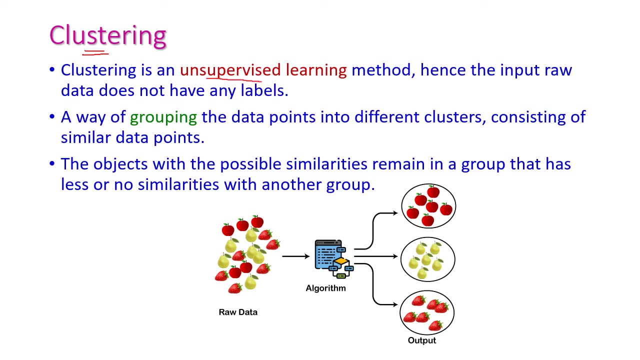 examples for regression: System of stability Amplification. tree regression, support vector regression. radial basis network for a regression Clustering. Clustering is an unsupervised learning method. The classification and regression will come under supervised learning method, isn't it? So the clustering is an unsupervised 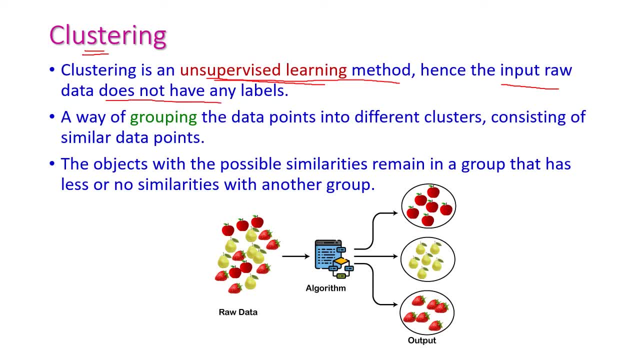 learning method. Hence the input raw data does not have any error label. this is called as plus frame, a way of grouping the data points into different clusters consisting of similar data point. so the similar data points will be grouped together to form the clusters and the objects with the 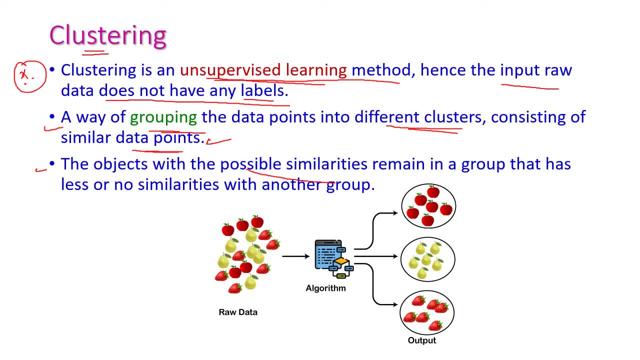 possible similarities remains in a group that has less no similar, that is, no similarities with other group. ok, for example, this is our raw data: here we are having a collection of fruits, and that data will be given to our plus string algorithm. the algorithm will separate all the data based on the similarities. 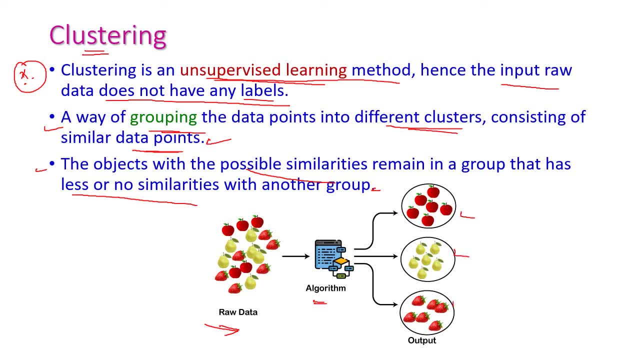 ok, so this will cluster, this will group all the fruits into different. different clusters are different groups. ok, and this is cluster ID 1.. Cluster 1, the ID is 1, this is 2 and this is 3.. Okay, these are the some of. 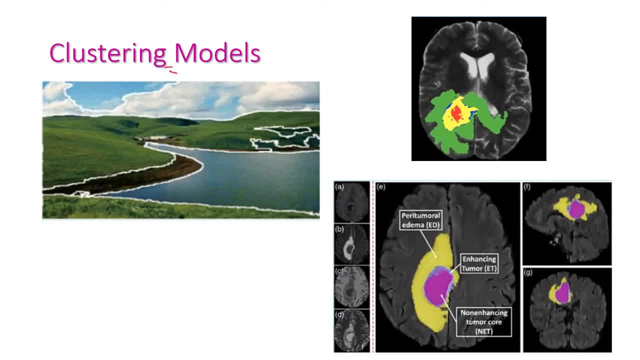 examples for clustering models. The first one is the natural scenario. Here the algorithm separates the water region, land region, grass region and sky regions. in this diagram. The similar data will be grouped together and that will be separated from this diagram. Okay, so this is called as clustering model. When come to next example, the affected region. 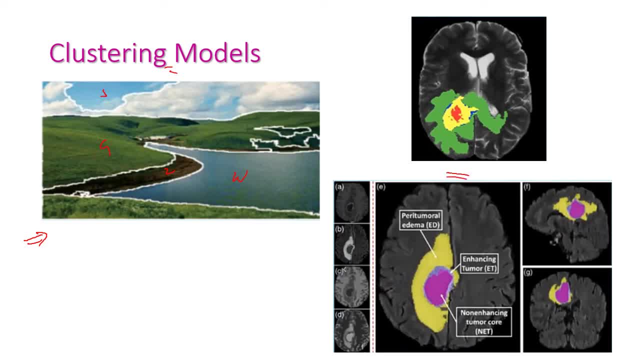 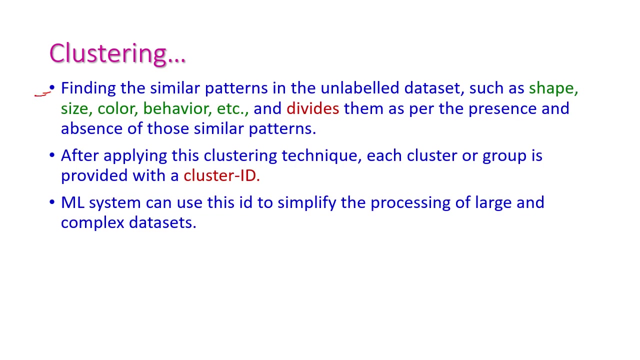 is separated from the normal region by the given diagram. Okay, so these are the medical images. From these medical images, we can easily identify the affected region from the normal region. Okay so, okay, These are the popular examples for clustering model. Okay, so here the clustering is used. 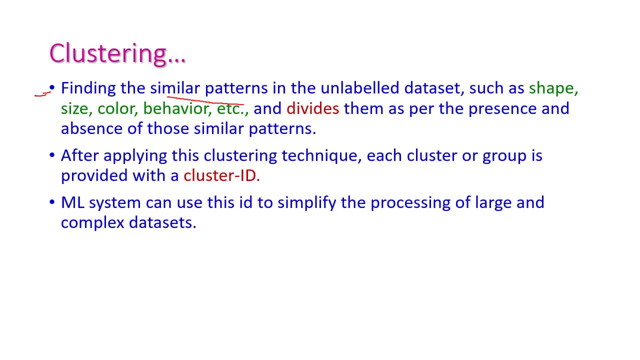 to find the similar patterns in the unlabeled data set, such as shape, size, color, behavior, etc. So, based on these attributes, the clustering algorithm divides the clustering model by the presence and absence of the similar patterns. After applying this clustering technique, 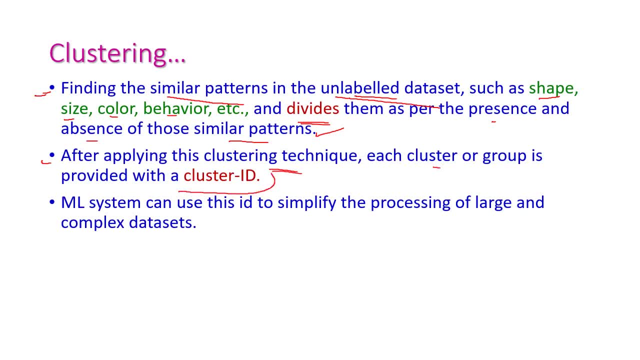 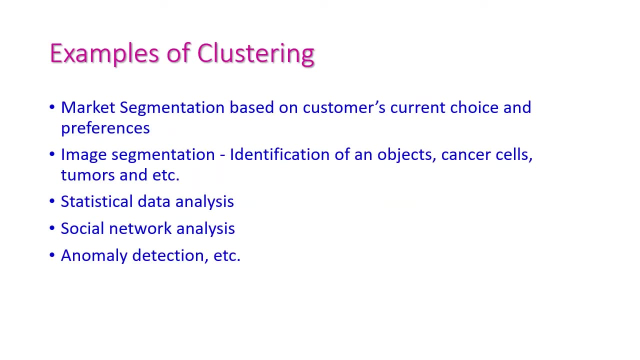 each cluster or group is provided with a cluster ID and the machine learning system can use this ID to simplify the process of large and complex dataset. Okay, so this is the first example. Here the clustering model divides the clustering model. clustering First one is market segmentation based on customer's. 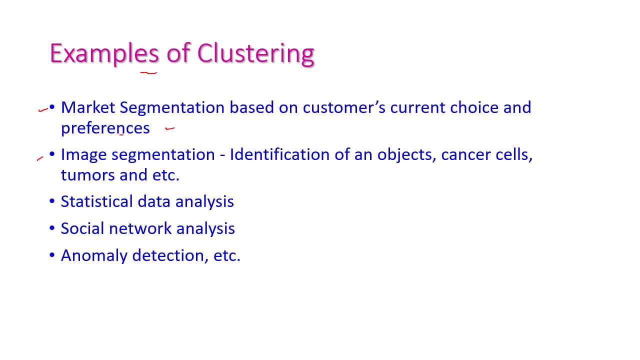 current choice and preferences. Second one: image segmentation, that is, identification of an object, cancer cells, tumors and etc. And next one is statistical data analysis, social networking analysis and anomaly detection, etc. And these are also other popular examples that will come under clustering. 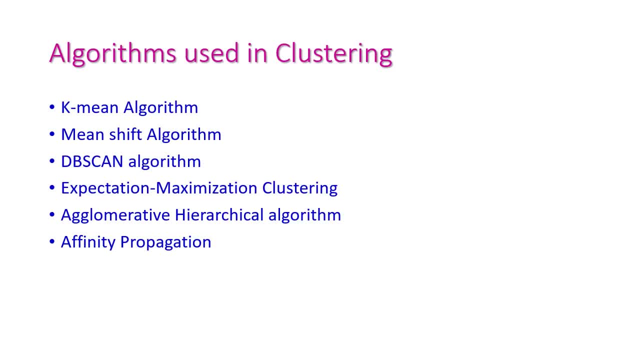 And the popular algorithms used under clustering are K-mean algorithm, mean shift algorithm, dB scan algorithm, expectation maximization, clustering, agglomerative hierarchical algorithm, affinity propagation. So these are the popular algorithms used in the Up to this. we have seen the